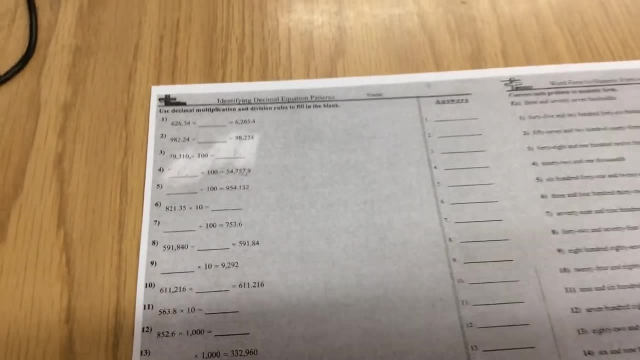 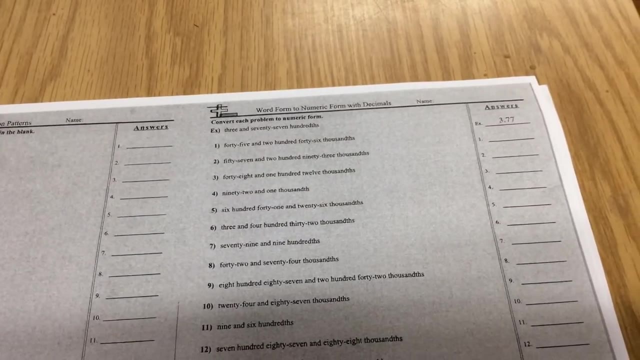 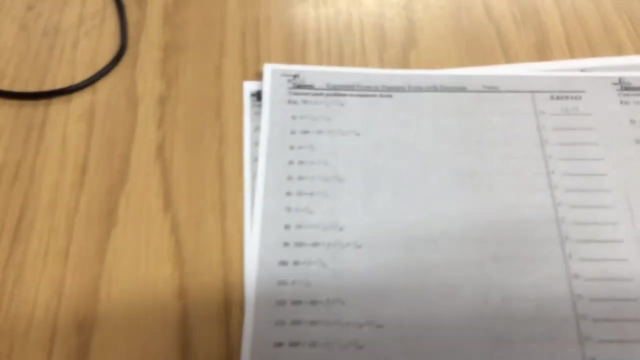 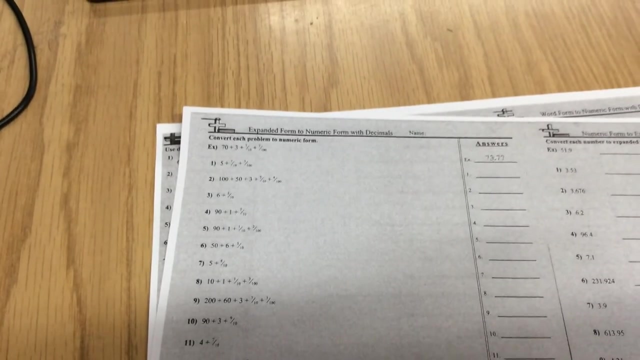 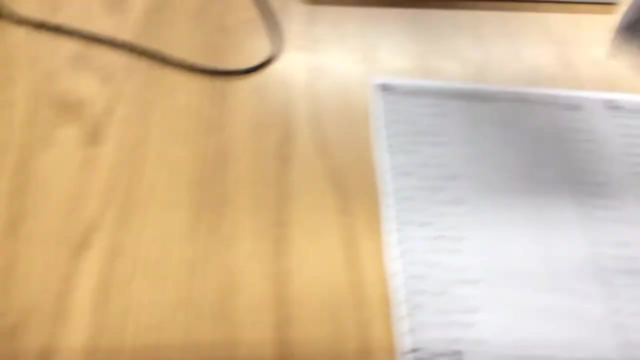 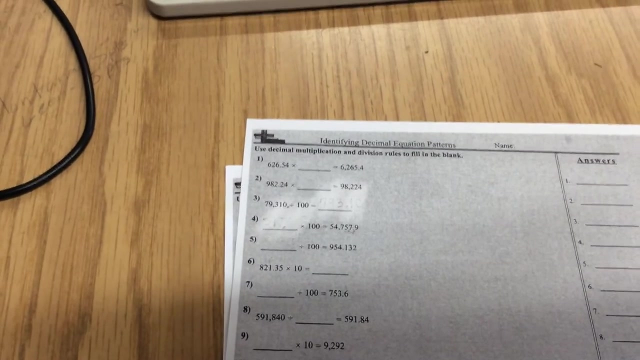 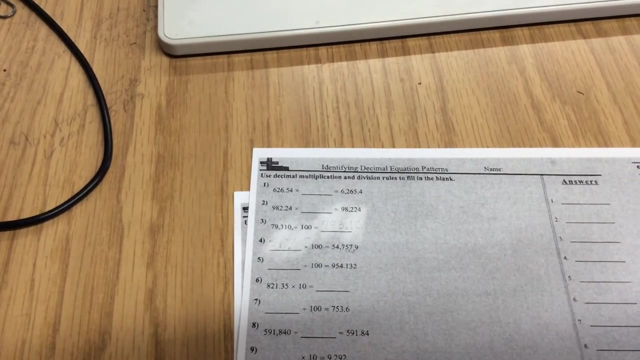 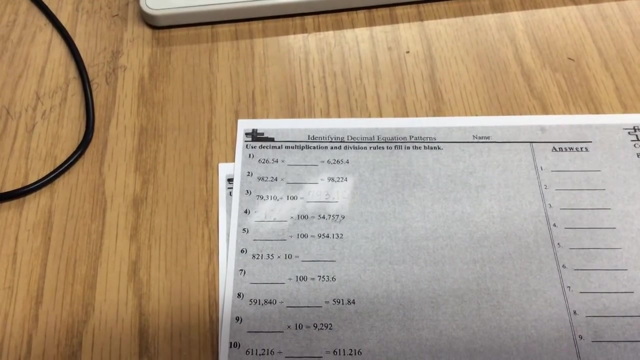 Okay, guys, this video we're going to be doing, identifying decimal equation patterns- Word form to numeric form with decimals. On the back side it has convert each problem to numeric form, So it's in expanded form with decimals, And then numeric form to expanded form with decimals. So we'll start and we'll do a couple Again. remember that any time you're multiplying a number, you're making that number larger. If you're multiplying or dividing by a power of 10 or a multiple of 10, the decimal will move to the right. You can count your zeros, You can use your exponent to tell you how many places to move it. 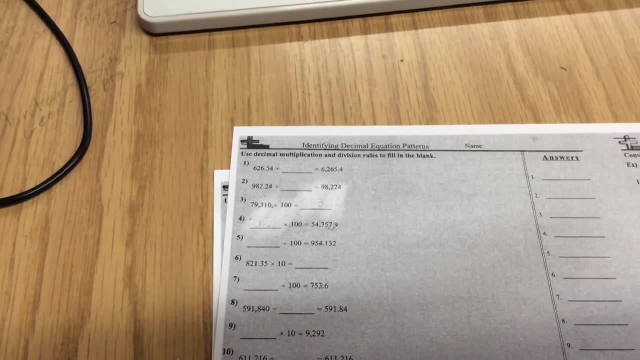 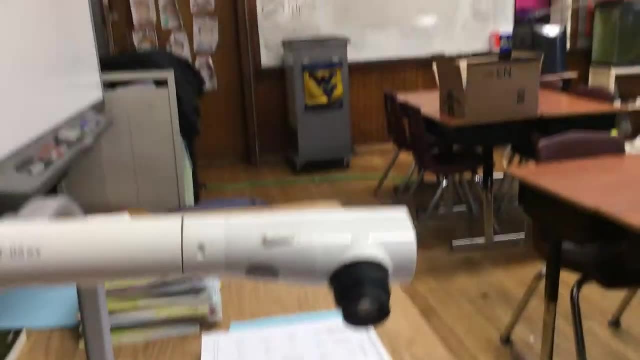 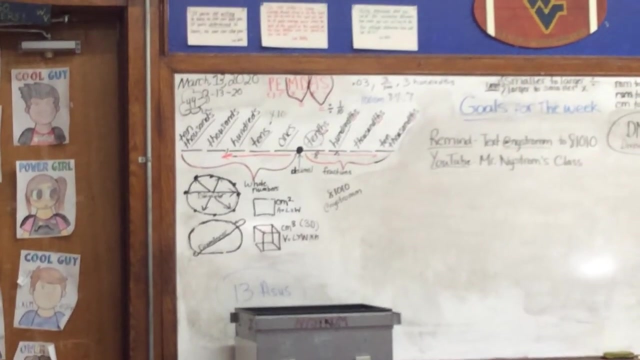 If you're multiplying, you move to the right, And if you're dividing, the decimal will move to the left, which will make the number smaller. Remember your place value. Again, there's the decimal. Remember the decimal also stands for: and in a sentence, in a number sentence in word form. 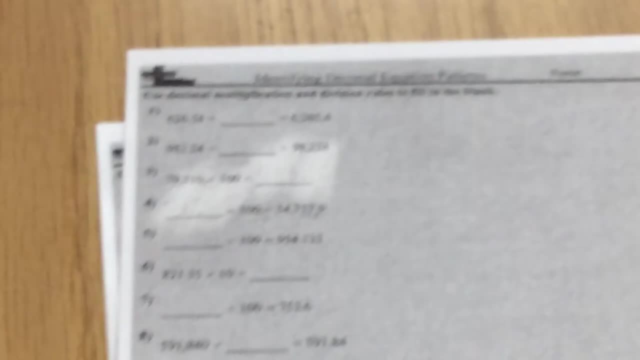 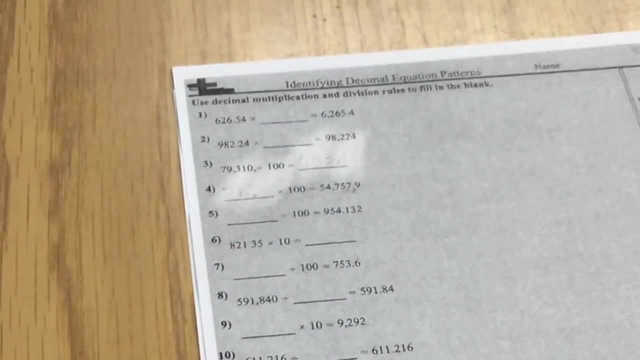 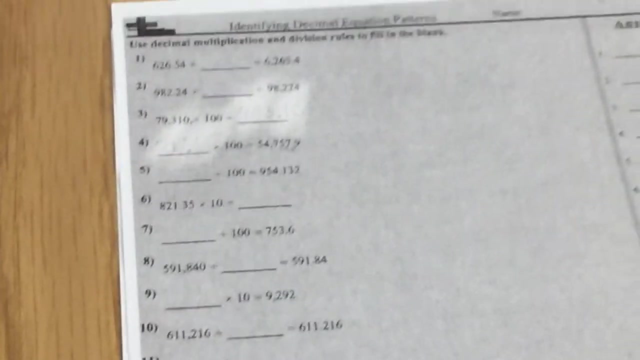 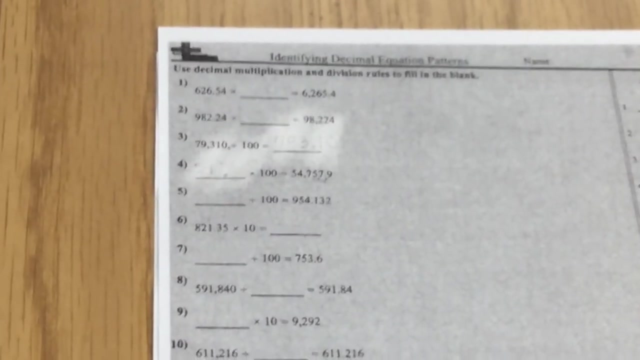 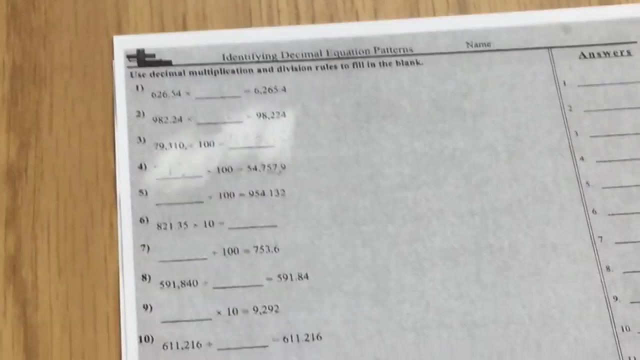 And we'll just do a few of these here. This seems to be the part that most of you are having trouble with. It is taking the decimal and multiplying or dividing by multiple of 10. And you have to find the missing number Now in the first one, or we'll actually start with having trouble getting into focus here. 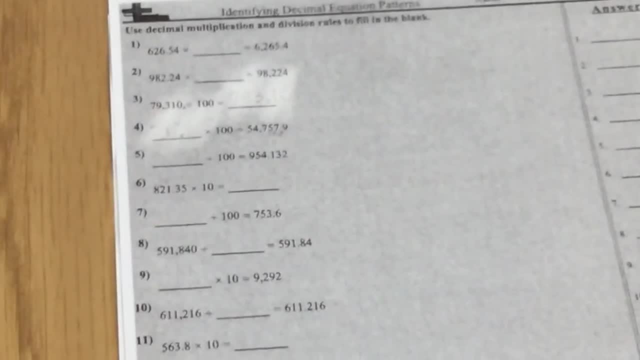 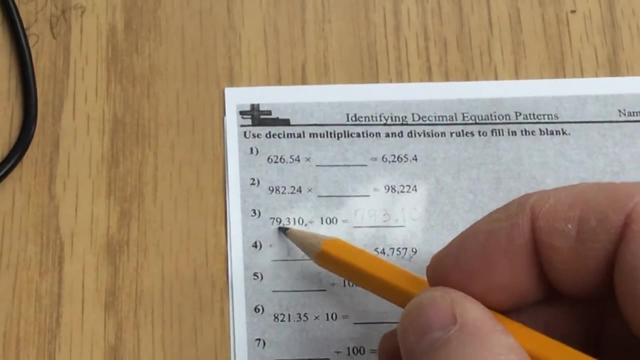 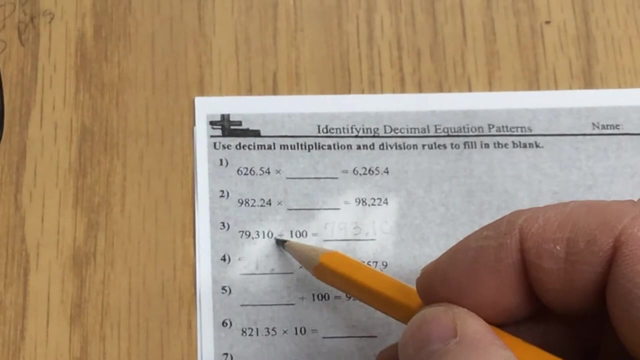 We have, we'll do number three. We have the number 79,000.. There's a comma, that's not a decimal: 310.. Now it's also important to remember that after any whole number there is a decimal, whether or not it's written or not. 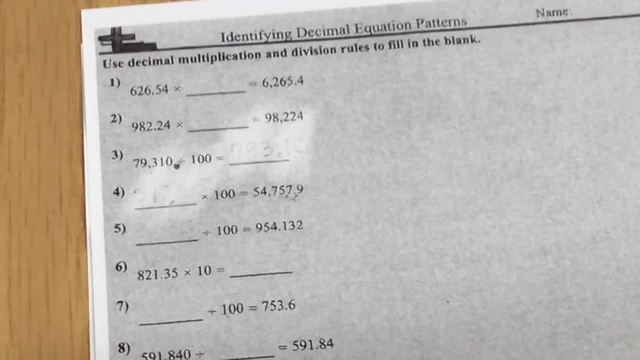 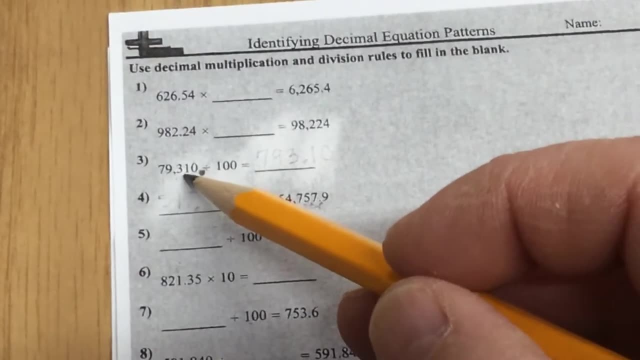 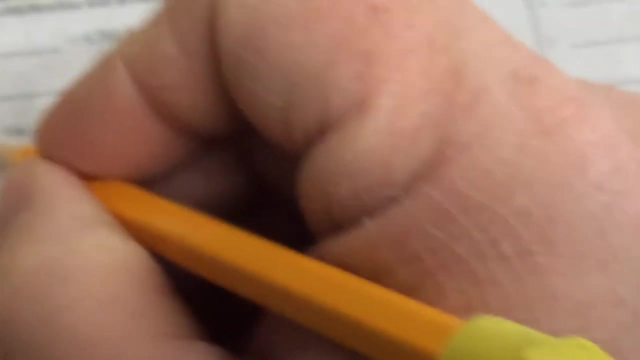 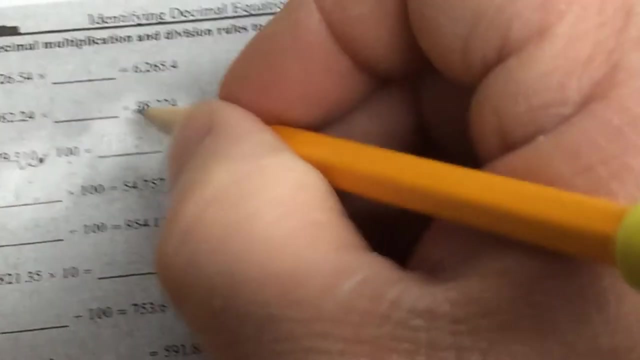 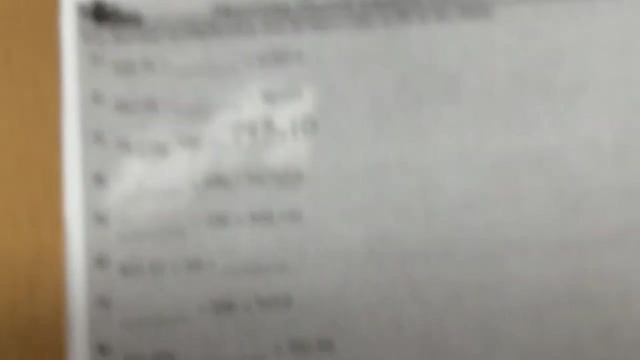 And we are dividing that by 100.. So that means we're going to make that number smaller By 100 times. So we're dividing this number up by 100.. So there are two zeros. So we are going to move that decimal two places to the left: One, two which would put the decimal now between the three and the one, which would give us 793. 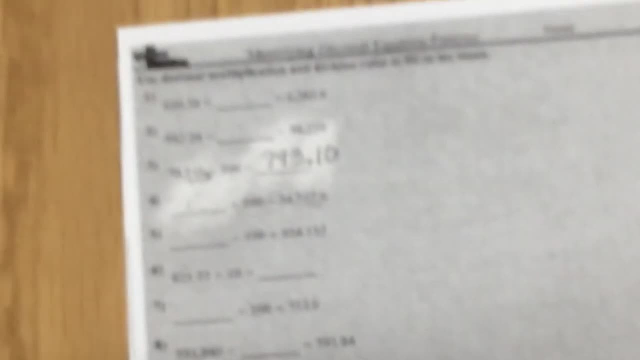 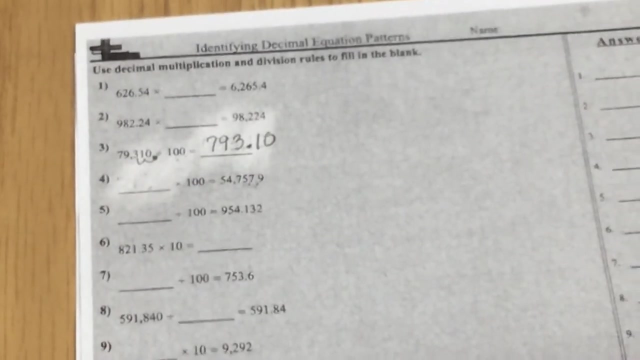 And one-tenth or ten-hundredths, which is the same. Okay, That zero on the end does not change the value, It just changes how you say it. Okay. So let's look at which is a smaller number. This is a smaller number than what we started with. 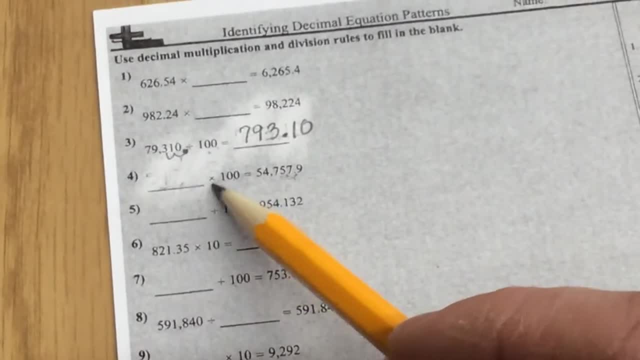 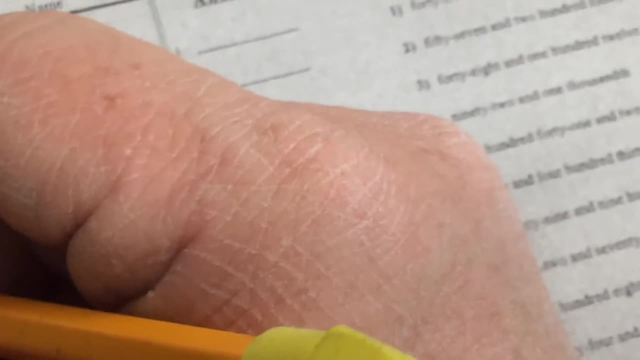 Now let's look at number four. We have some number that we've multiplied by 100. And we got this number. Now the decimal is- and I know this is kind of hard to see, but the decimal is right there between The seven and the nine. 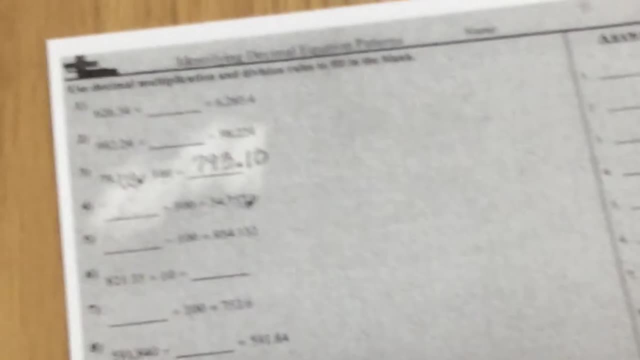 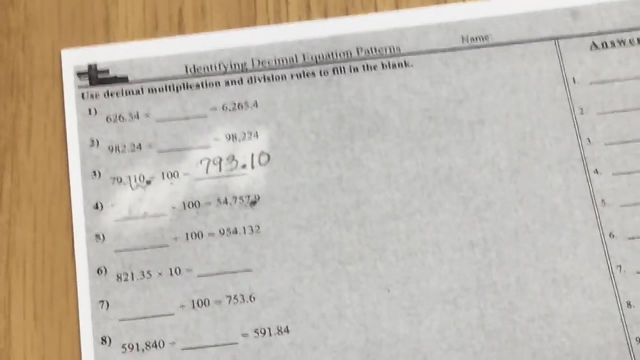 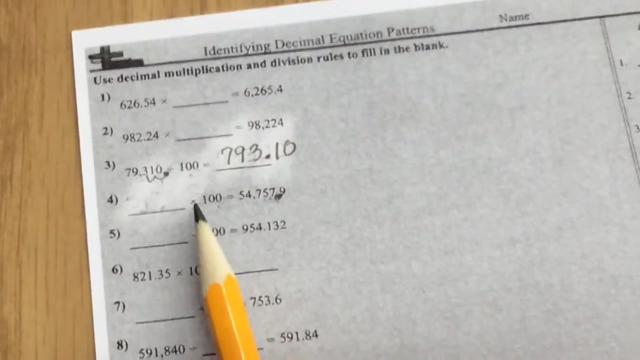 I made that kind of big so you could see it. Okay, So we have 54,757 and nine-tenths. Now that's what we ended up with after we multiplied by 100.. So to find what we started with, remember the reverse of multiplication. the opposite is division. 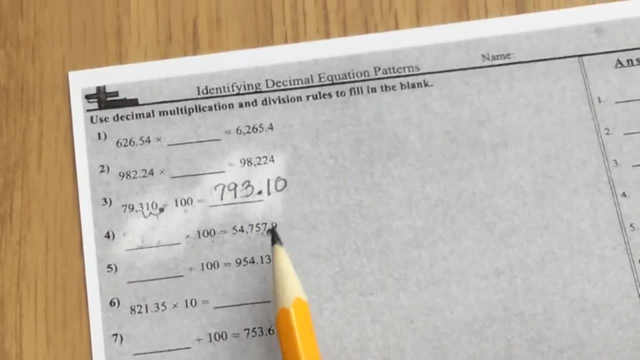 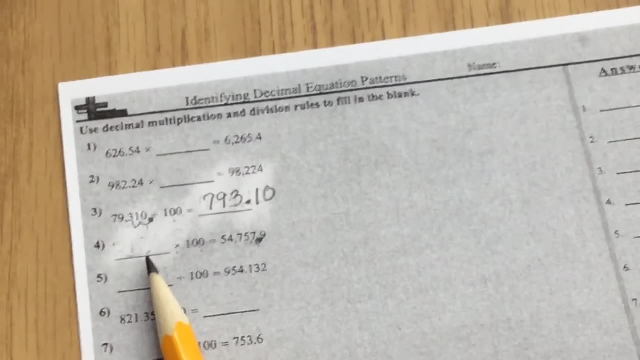 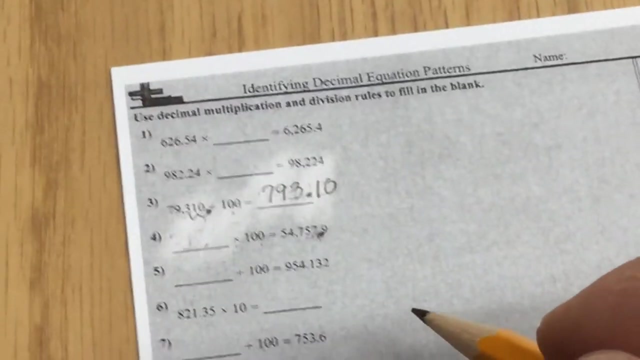 So to find what we started with, we can simply work backwards And divide this number that we ended up with by 100, and that will give us what we start with, So let's move that decimal. if we're dividing by 100, there's two zeros, so let's move two places to the left. 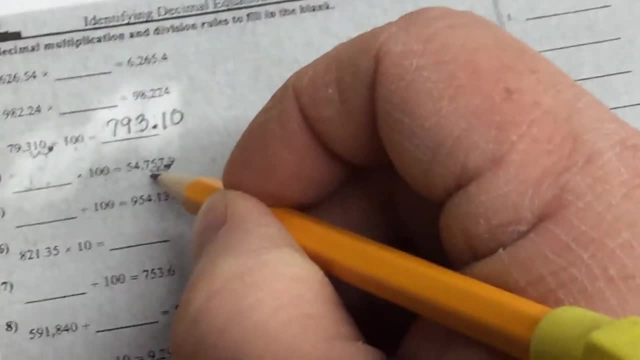 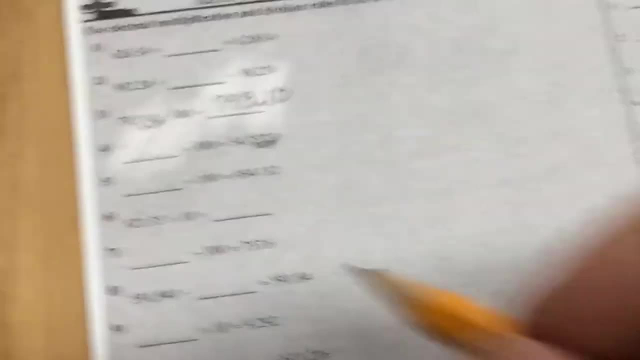 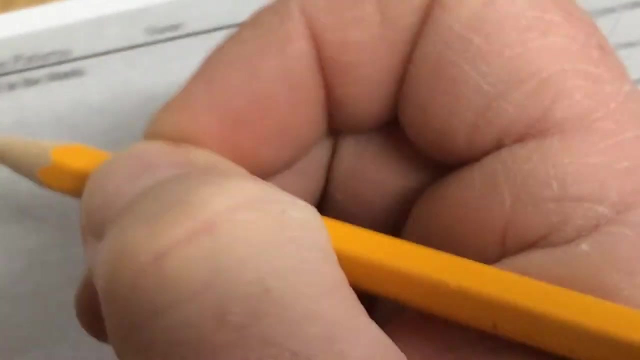 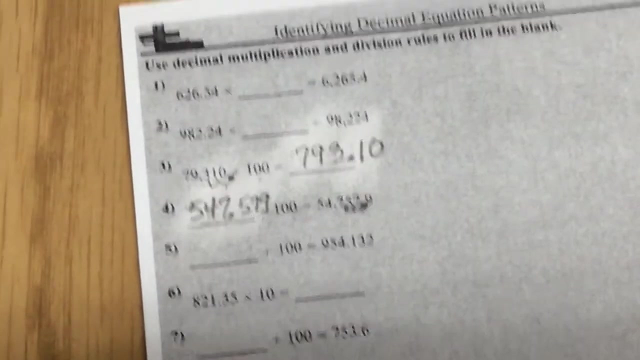 One, two. So now our decimal is between the seven and the five, Which makes what we started with. we have five, four, seven, decimal five, seven, nine. Now if we started with that number, now you can look and check and work your problem the right way now 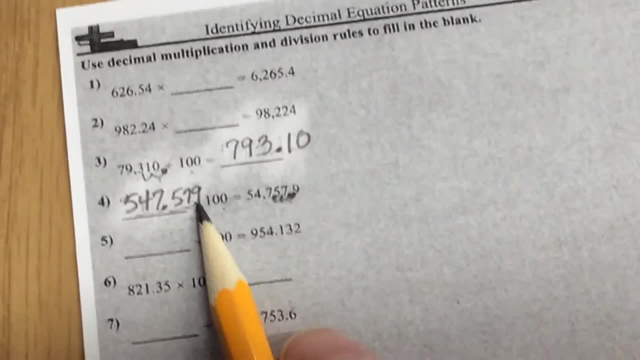 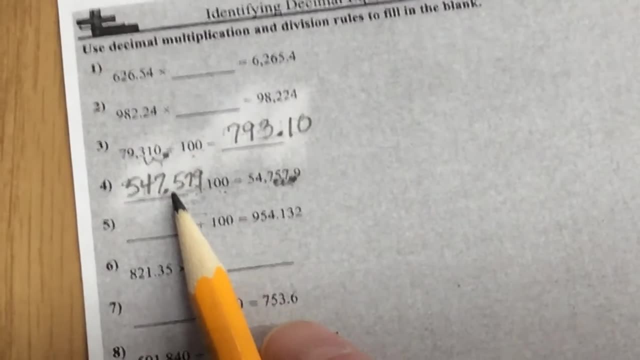 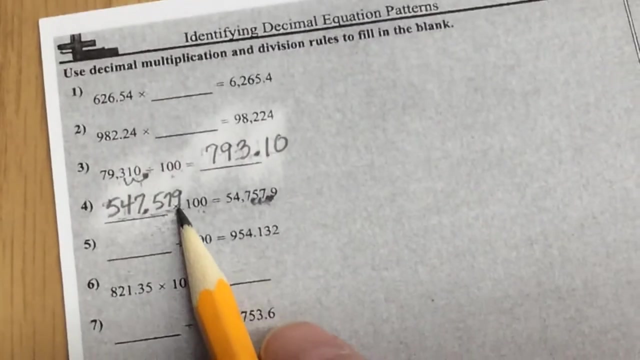 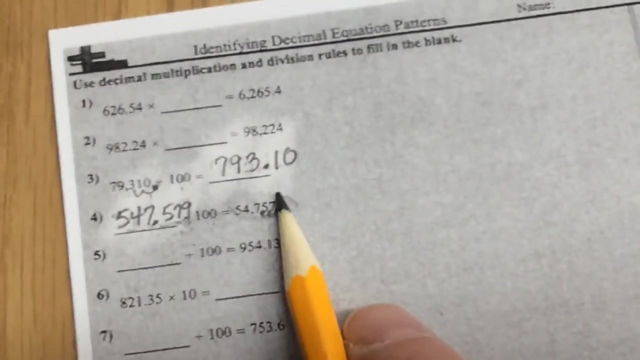 547 and 579 thousandths, We have tenths, hundredths, thousandths times 100. So that means if we're multiplying, we're going to make this number larger And we're going to move to the right one, two spaces. so that would put our decimal back between the seven and the nine, which is what they had for us here as our product. 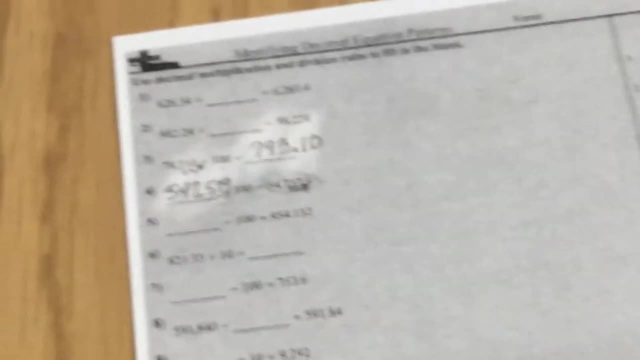 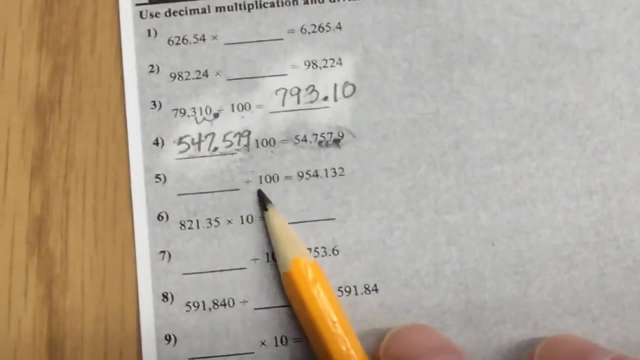 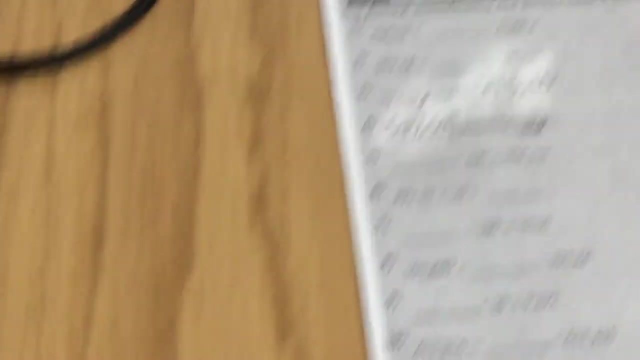 So you can simply work backwards and do the opposite to find your starting number. Same thing for number five. we have some number that we divided by 100, and we got this number. Okay, I'm going to try to hold this still, so you can see. 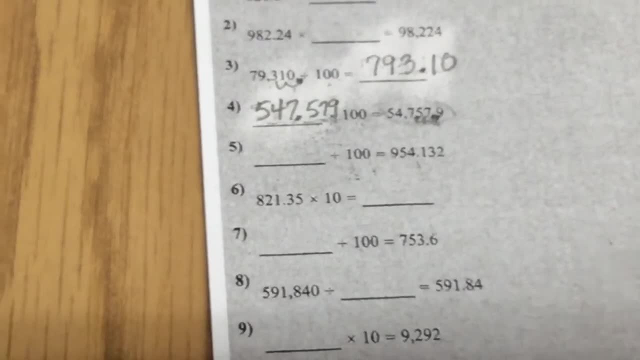 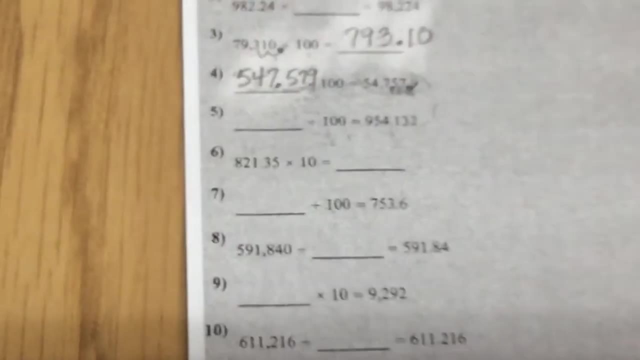 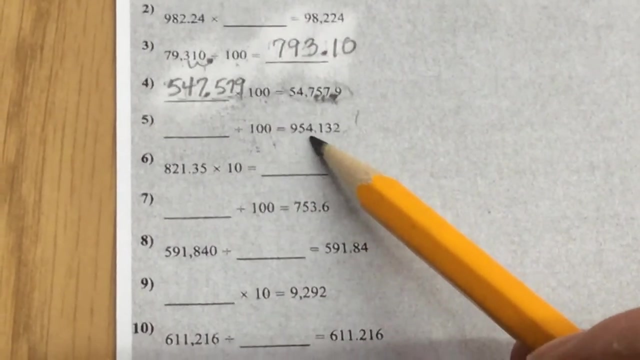 Kinda hard. So we have 954 and 132 thousandths. There's our decimal between the four and the one So we can work backwards. So we took a number and made it smaller by 100 times and got this. So we know our decimal is going to need to move to the right. 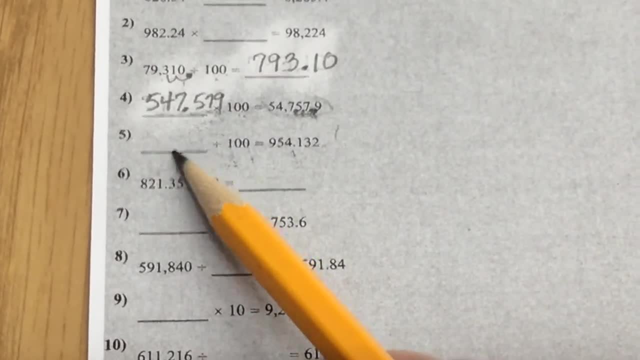 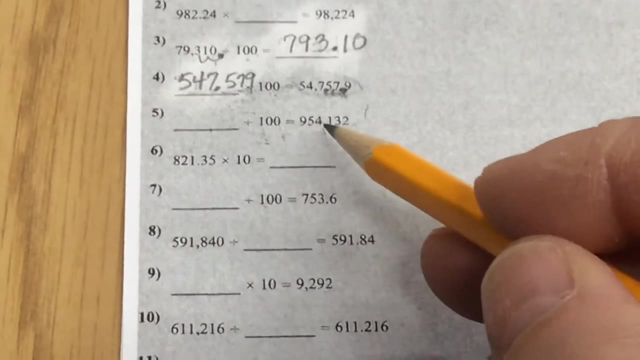 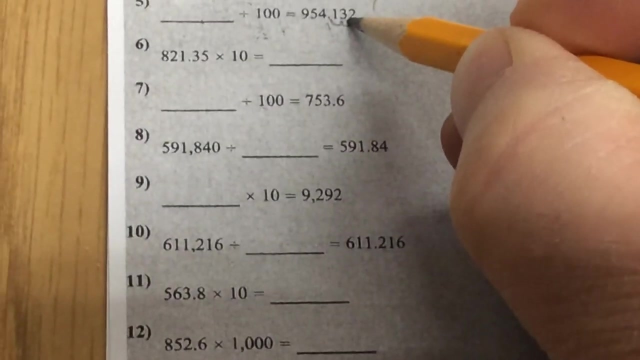 to make it smaller, Right To make it smaller. get a larger number over here that we started with. So there are two zeros instead of division. we're going to work opposite and we're going to multiply this number by 100, so that would put our decimal between the 3 and the 2.. So over. 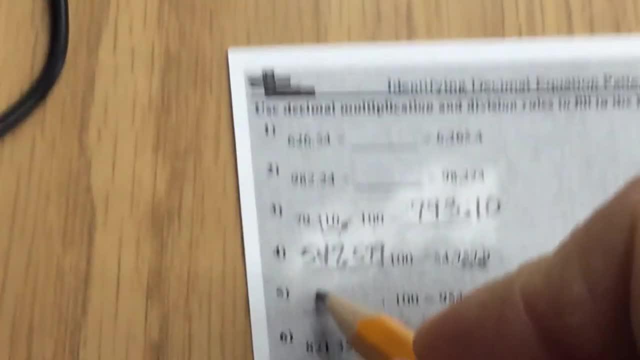 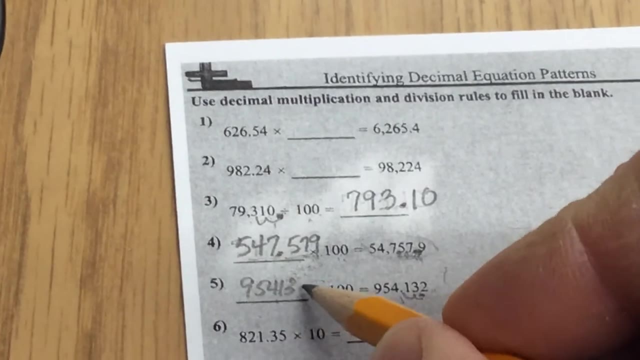 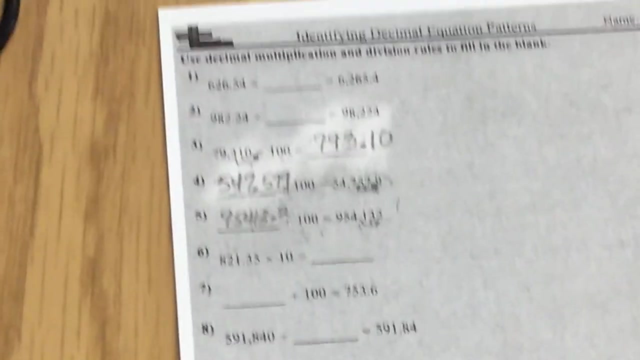 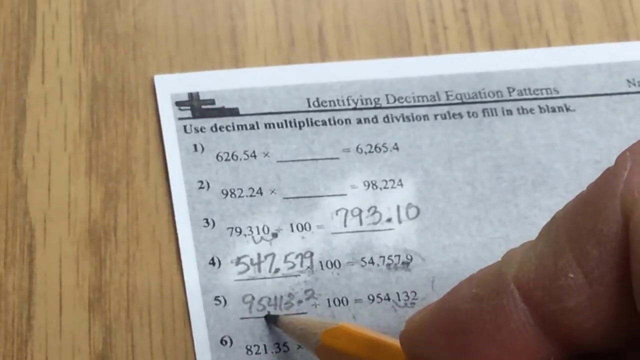 here what we start with: 9, 5, 4, 1, 3, decimal 2.. I know there's not a whole lot of room on this paper to write that, but we have, and we can put our comma in between every three numbers, remember that's. 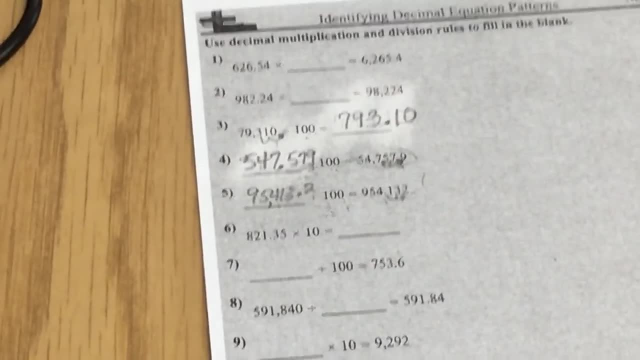 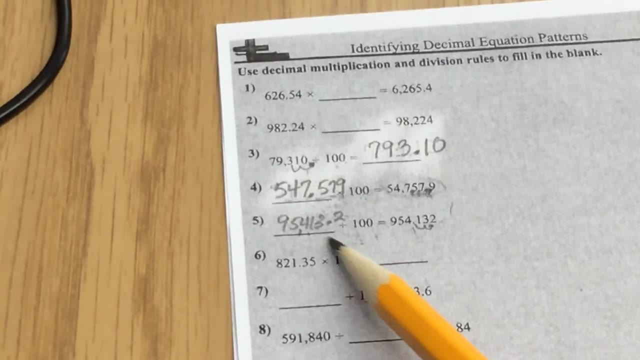 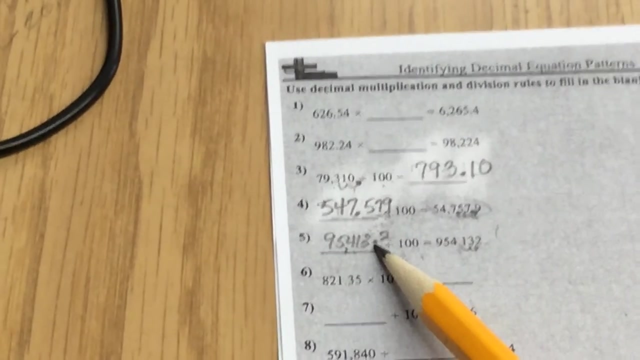 every three numbers. So we have ninety, five thousand four hundred thirteen and two tenths. now if we take that number and divide that by 100- remember our decimals here- divide by 100- we move to the left if we're dividing. so if we move one, two, that would put our